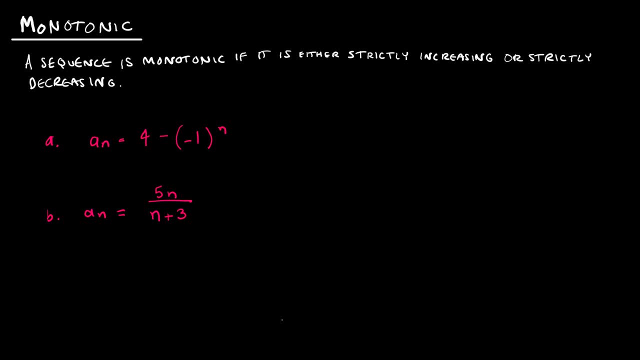 concept. The first concept is monotonic, and monotonic sequence just means that it's continually increasing or non-decreasing, and it's or continually decreasing or non-increasing. So essentially what we're saying is: a sub 1 has to be less than or equal to a sub 2,. 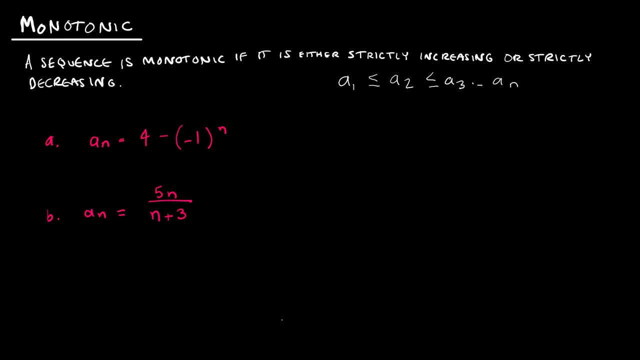 less than or equal to a sub 3, all the way through a sub n, Or obviously it could go in the opposite direction. The key here is that you're never going to have a value that's bigger than the next and then less than the next, because that would not be. 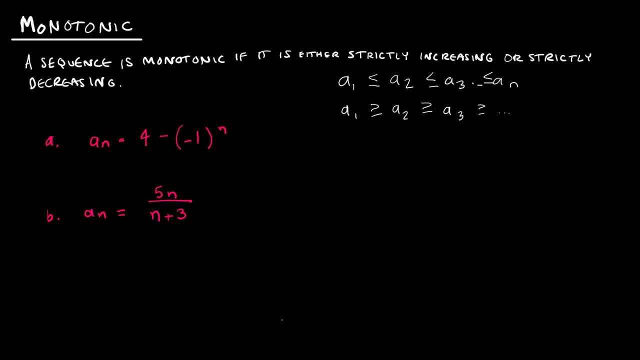 monotonic Oops. So we get the idea that it's either continually increasing or continually decreasing. So that's what we're going to do first is just take a look Now. you can obviously reason through these. You can say: well, what's going to happen here? Negative 1 to the n. 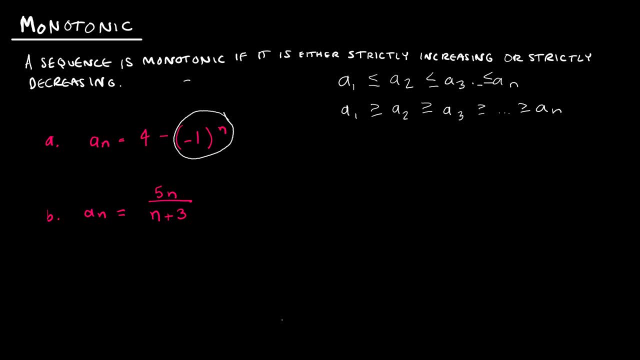 we've talked about this already. We know that this is going to be a negative 1, and then it's going to be a positive 1 and a negative 1 and then a positive 1.. And so it's constantly increasing and decreasing. So we get the idea that it's either continually increasing 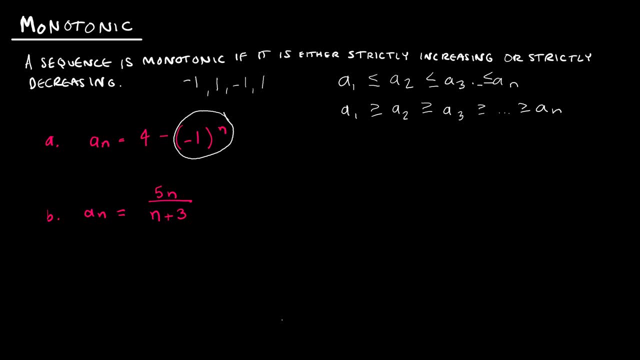 or decreasing. So it's clear, before I do any kind of work at all, that if I take 4 minus negative 1, 4 minus positive 1, that's not going to be strictly increasing or strictly decreasing. But remember that you can always just do the work and actually, you know, figure out the first few. 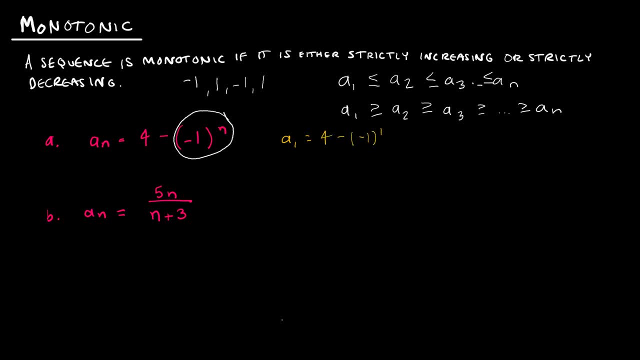 terms to find the pattern. So 4 minus negative 1 to the first. we already said, that's going to be 4 minus negative 1, which is going to be 5.. And then a sub n to the n, which is going to be 5.. 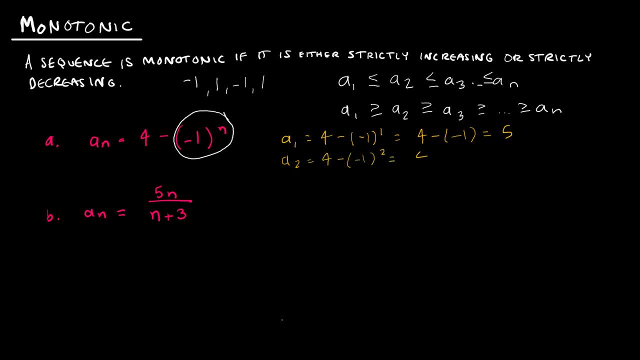 Sub 2, 4 minus negative 1, squared which is 4 minus 1,, which is 3.. And then a sub 3, 4 minus negative 1 to the third. negative 1 to the third is negative 1, which gives me 5. And we can see. 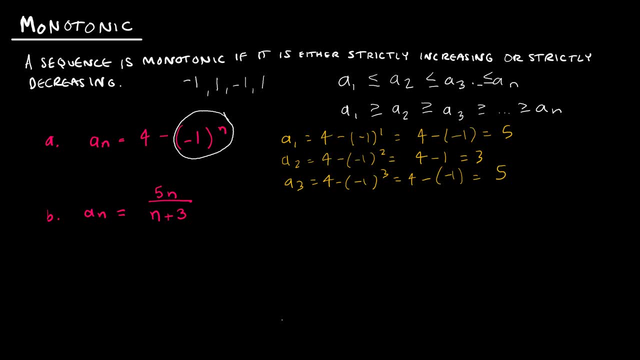 that this is going to be an oscillating function. It's going to go back and forth between 5 and 3 and 5, and 3 and 5 and 3. And it's just going to keep happening. So this is not monotonic. 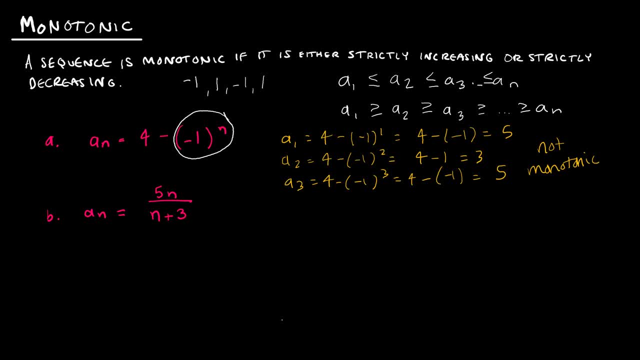 Because it's not strictly increasing or strictly decreasing. It decreased, then it increased, And then it's going to decrease and then it's going to increase. And again, we call that an oscillating function if it oscillates back and forth between 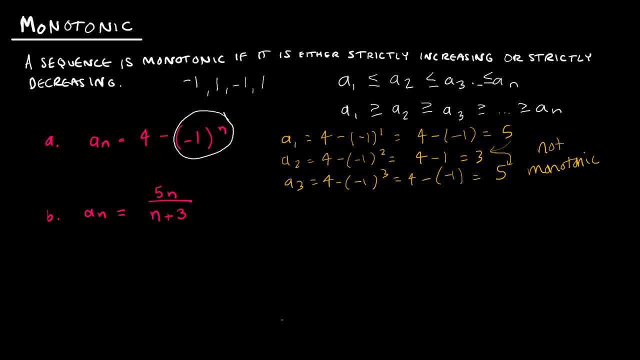 different values. Now let's take a look at example B And again, feel free to either find the values and see the pattern, or you can reason through it. So let's just find the values first. This would be 5 times 1.. 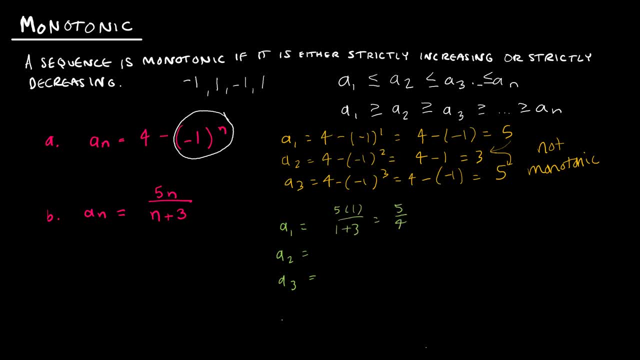 Over 1 plus 3,, which would be 5 over 4.. So just a little bit over 1.. A sub 2, 5 times 2, 2 plus 3.. That's 10 over 5, which is 2.. So obviously that increased. Now let's see what's going to happen. 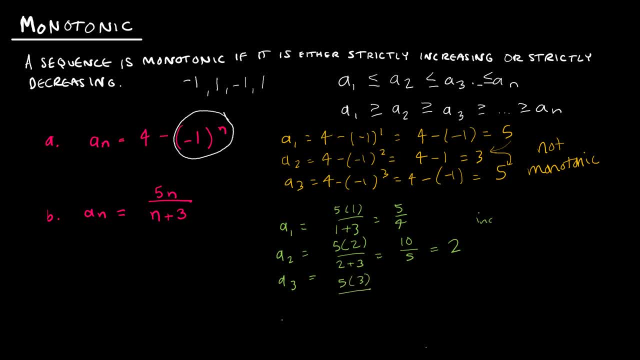 with a sub 3.. 5 times 3 over 3 plus 3, which is 15 over 6.. 15 over 6 is the same as 15 over 6.. So I can see that the value is going to increase And I can keep finding as many values as I need. 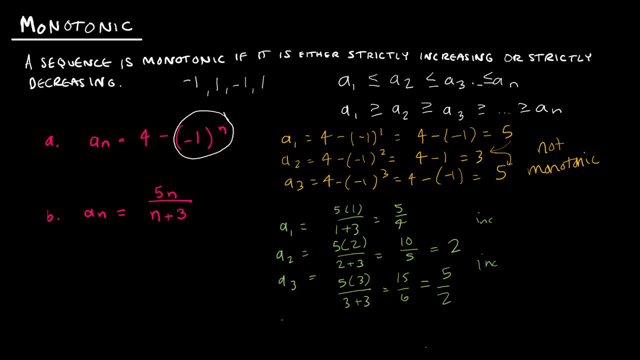 in order for me to be convinced. But, as I can see, this value is growing at a higher rate than this value, So this number is going to keep getting bigger, And so is this number, But this is going to get bigger, faster, And so it's very clear that this is going to continue to increase. 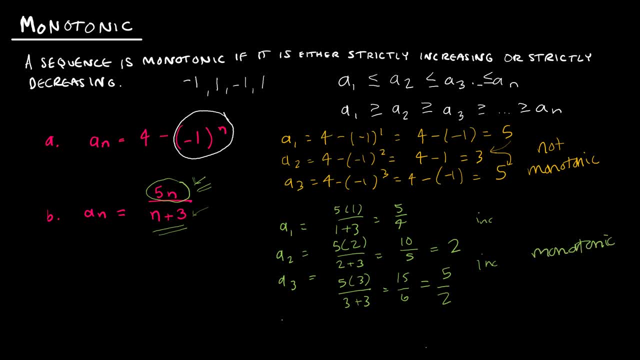 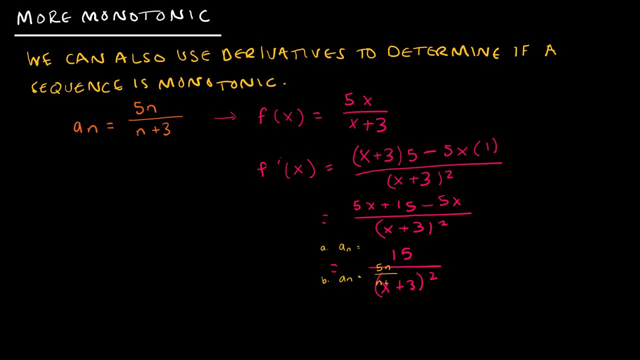 So this is monotonic. Keep in mind that we also know how to find the derivative of a function. So, using example B from our last slide, looking at the sequence of 5n over n plus 3.. Remember, I can look at that as: 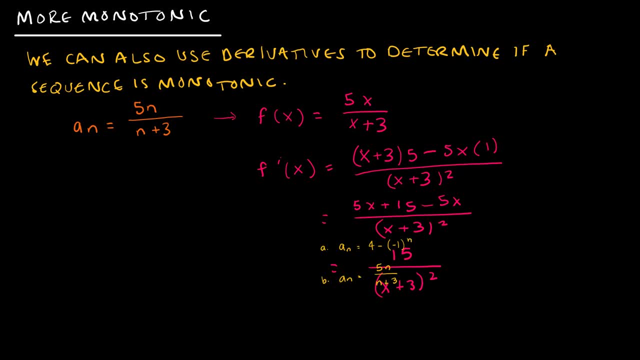 a function, f of x equals 5x over x plus 3.. And I can find the derivative of that function. And you can see, I've just used the quotient rule there And I have found the derivative. Now why is the derivative helpful? Because we know that the first derivative of a function 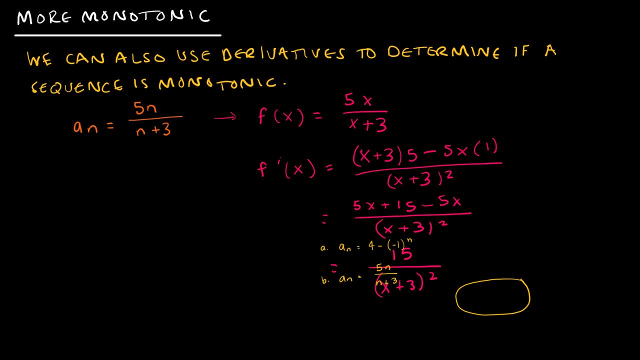 tells us if that function is increasing or decreasing. So if the function is positive, then it's increasing, And if the function is negative, then it's decreasing. By finding the derivative of this function, I can see that no matter what I plug in for x, it's going to be. 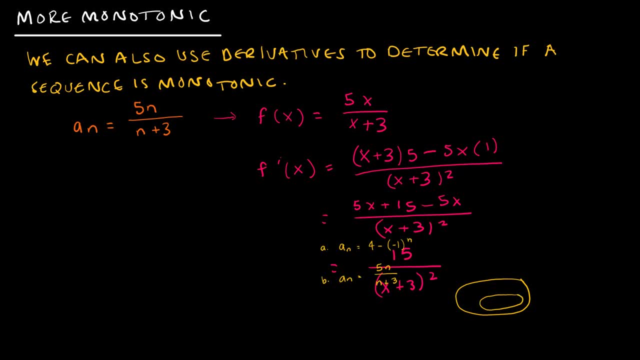 squared. So I've got 15 over some positive value, And 15 over a positive value is always going to be positive. So, because this is always positive, this is always increasing And therefore it's monotonic. The other characteristic we need to talk about is: 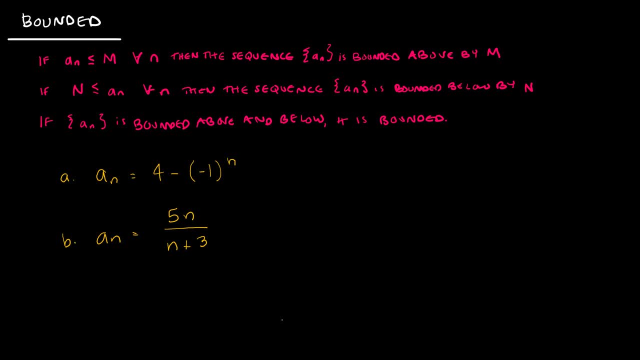 whether or not a sequence is bounded, and it can be bounded above, bounded below, or bounded both above and below, which we would just call it then bounded. So, looking at our first example from our previous slides, remember that this oscillated between five and three, And so this is obviously 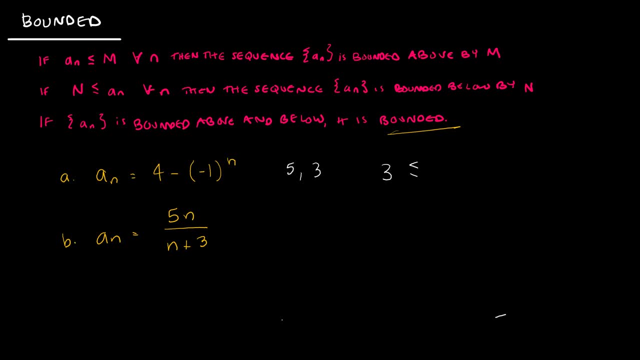 bounded, both above and three. So this is what causes the delineation of 2 here, which is a above and below, because we could say: 3 is less than or equal to a sub, n is less than or equal to 5.. In our second example this is also bounded, so this is called bounded because it was bounded. 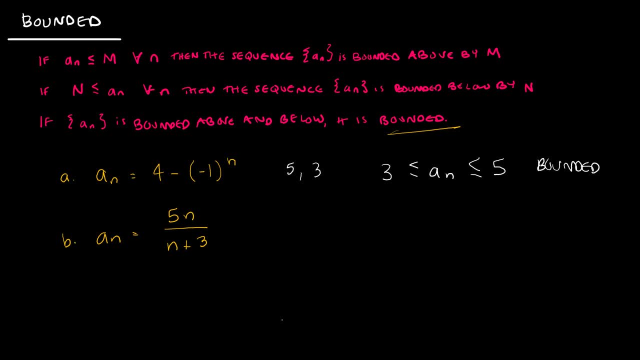 both above and below. In our second example, remember, we found 5 fourths and then we continued and we didn't ever find an upper bound. but if we continued- and it would take us a while to get there- if we continued- we would find that 5 fourths is obviously the very lowest that we 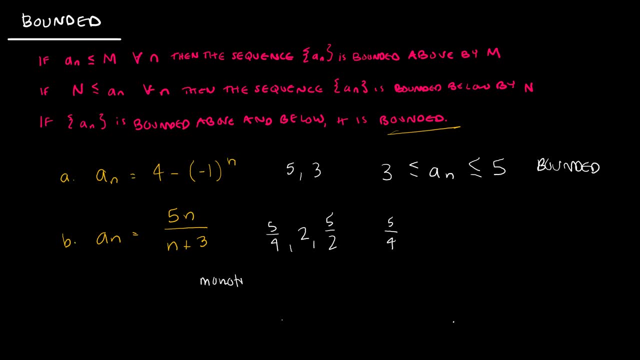 could get, because we decided this was monotonic. so it's continually increasing- Oops, I think I spelled that wrong: Monotonic- And if we continued and continued and continued, we would find that this gets continually closer to 5.. So this is also bounded. It is bounded above and below. 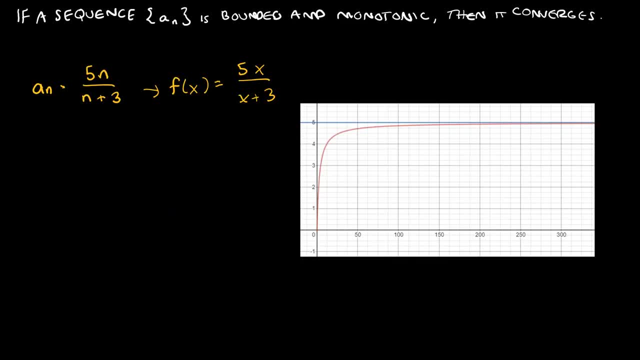 So the very last theorem that I wanted to talk to you about in section 9.1 then is theorem 9.5. that essentially says, if you have a sequence that is both bounded and monotonic, then it converges. So let's look at that before we actually look at our example. If we know we have a function that 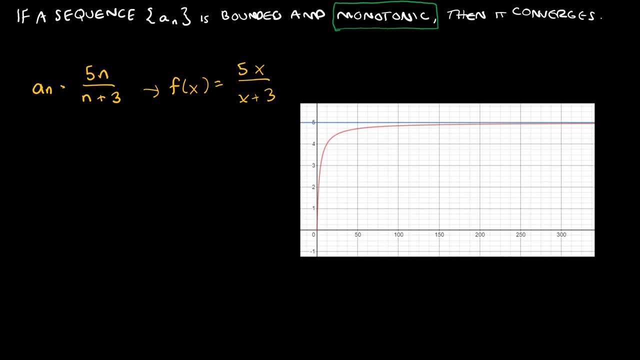 is monotonic, or a sequence that is monotonic, remember. monotonic tells us that it is going to continually increase, increase, increase or decrease, decrease, decrease without end. Now, if it's also bounded, that doesn't mean it's going to stop increasing. That just means.